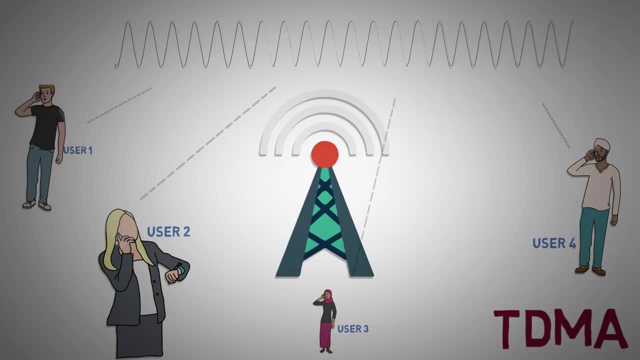 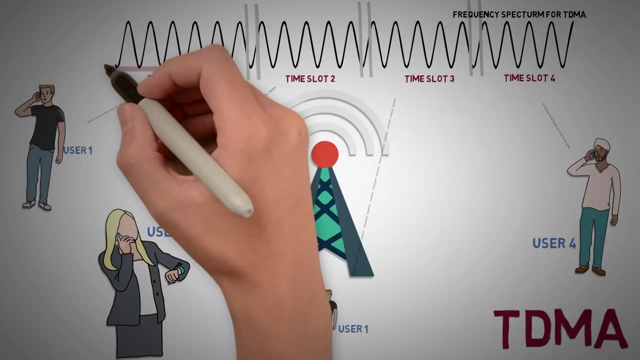 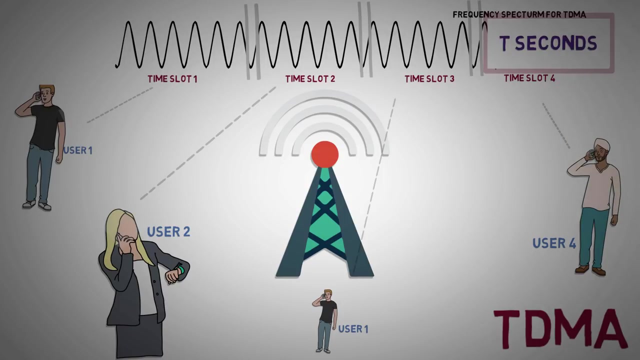 kilohertz TDMA which uses time division. multiplexing allows multiple users to share a common frequency band by allocating different time slots. Thus an in-channel TDMA where each channel is given a time slot of two seconds. signals coming from each user will be transmitted at intervals of in- into two seconds. 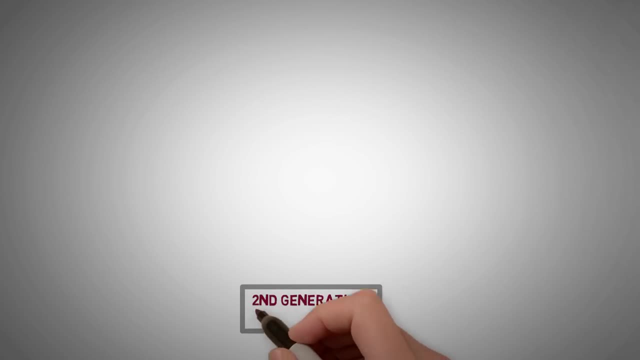 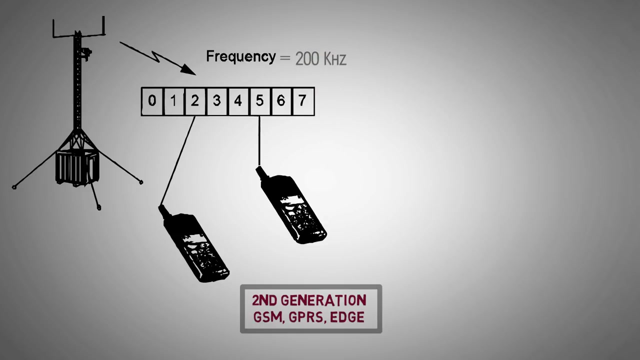 This technology was used in the 2G systems like GSM, GPRS and EDGE. Each user was provided one of eight TDMA slots in a bandwidth of 200 kilohertz. Dynamic resource allocation meant more users could be supported, but each channel could support only eight active users at a time. 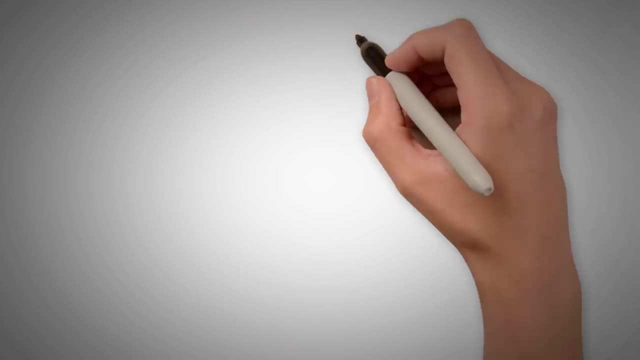 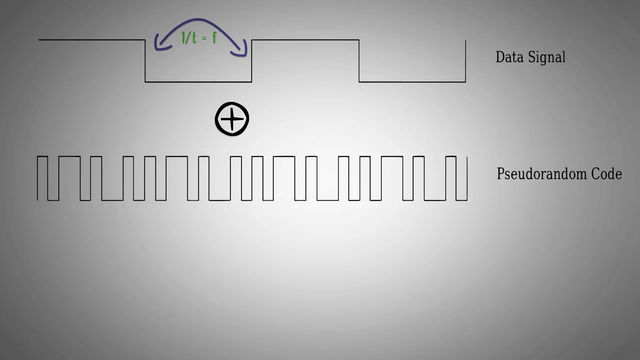 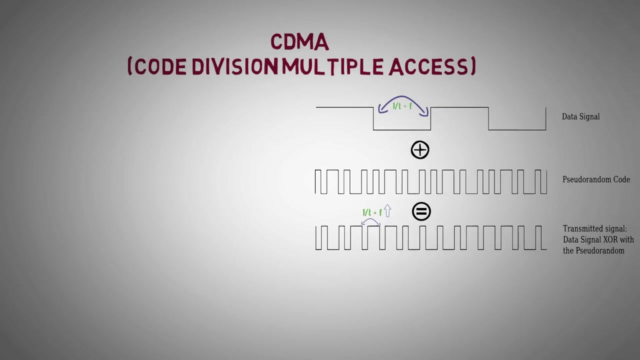 CDMA based on code division. multiplexing is a technique in which the data bits are modulated by a high frequency orthogonal sequence of bits, such as Walsh codes, or pseudo random codes, such as gold codes, to spread the signals over a large frequency band. Multiple such signals from different users are then transmitted over the same frequency. 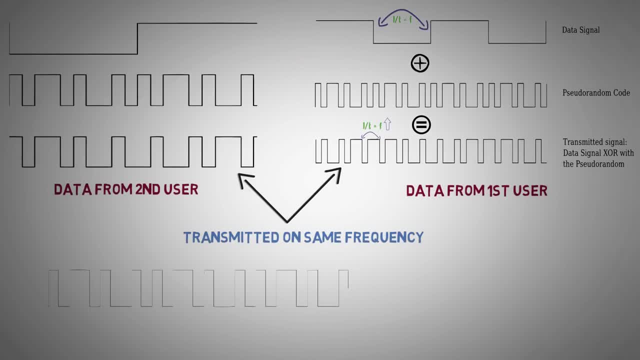 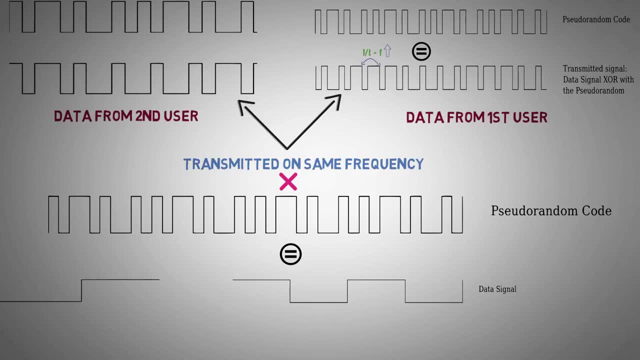 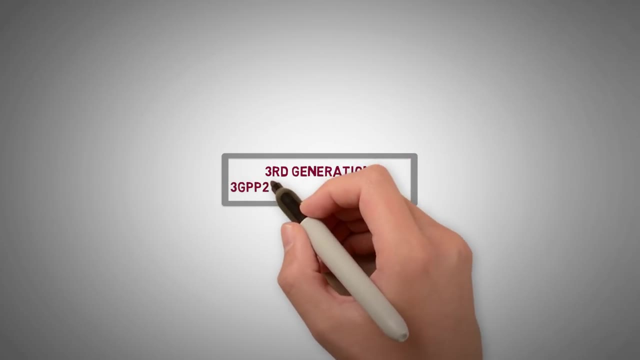 band. In order to retrieve, the signal receiver must have the same spreading sequence, which is multiplied to this composite signal in a process called de-spreading. This makes CDMA very secure and robust. It was used in 3GPP2 standards such as CDMA and CDMA evolution data optimized standards. 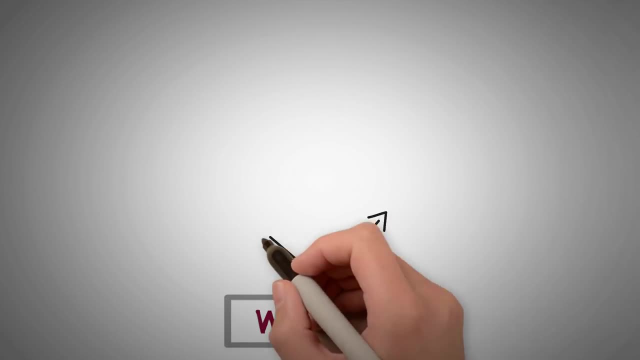 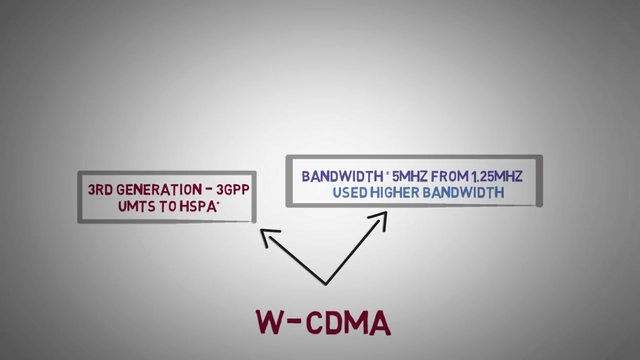 Wide band CDMA, or WCDMA, spreads the signals over a even higher bandwidth. This was used in the 3G standards of 3GPP, from UMTS to HSPA+, Where the available bandwidth was 5 MHz, Compared to 1.25 MHz used in CDMA. 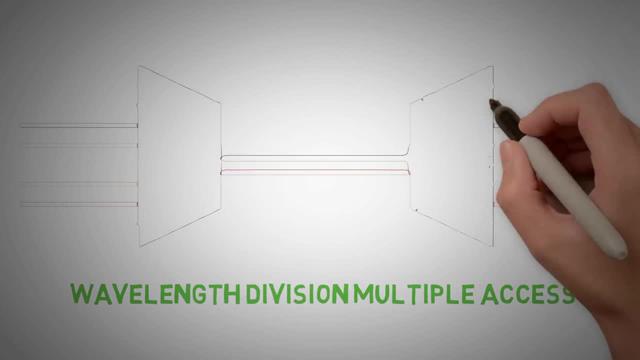 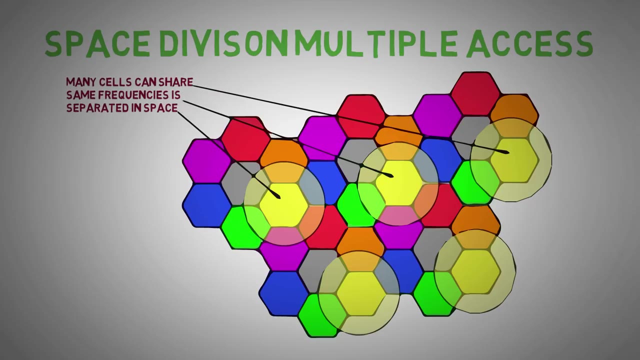 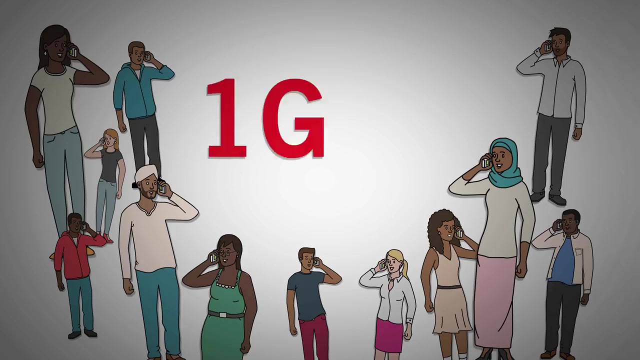 There are other multiple access techniques like wavelength division multiple access, which is used in fiber optics, and space division multiple access, which refers to spectrum reuse over non-overlapping areas. As the number of users and their demand started growing, communication networks evolved from 1G to 4G. 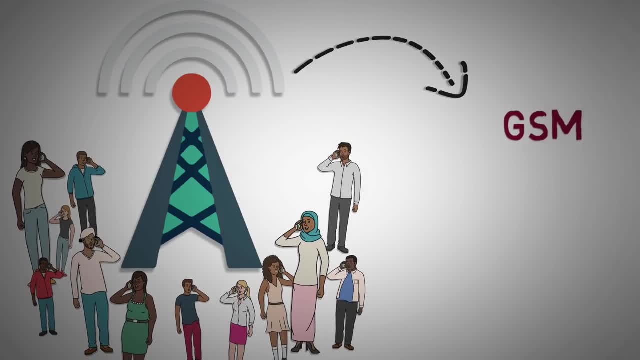 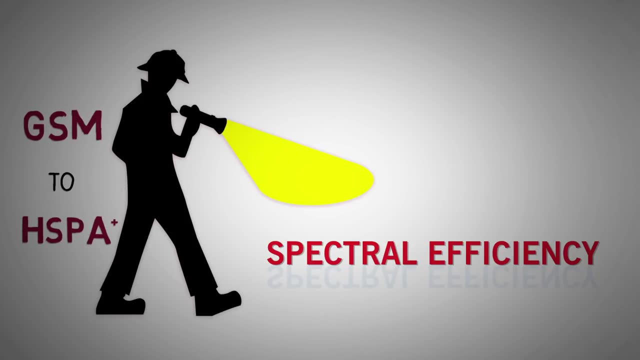 Radio part was significantly enhanced from GSM to HSPA+. This was used in 4G. Now focus was shifted towards better spectral efficiency by using higher modulation order like QPSK, 8PSK, 16COM, 64COM, etc. 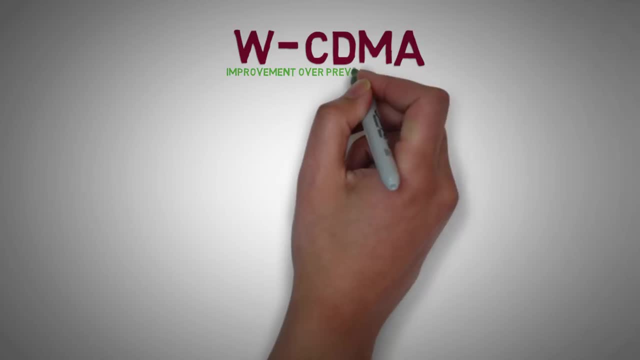 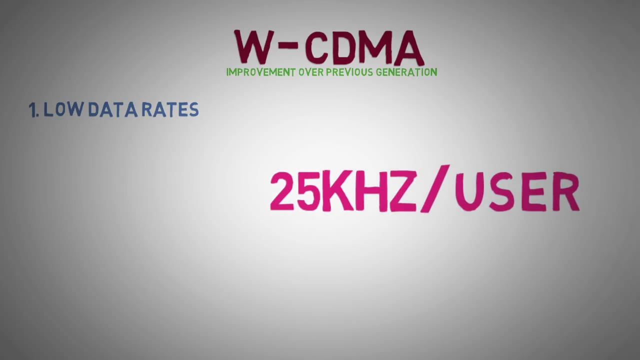 WCDMA improved upon some of the problems of earlier generations like, first, low data rates. in GSM, effective bandwidth for a user was only 25 kHz. Second, congestion at peak hours. As the frequency, chunks and time of the signal were reduced, the frequency of the signal. 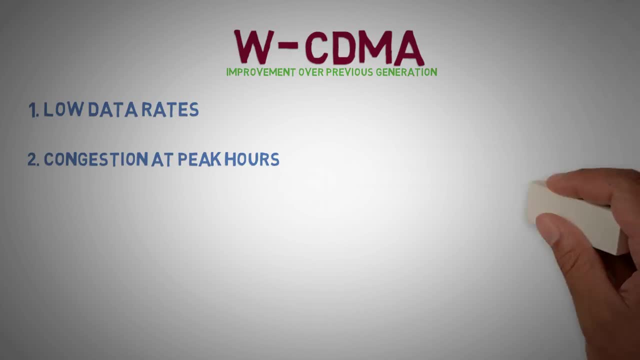 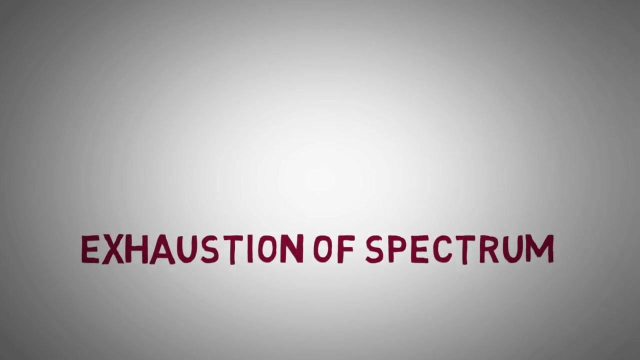 chunks and time slots were very limited. Third, resource wastage. Resources remained idle when users were inactive. Fourth, poor spectral efficiency due to guard bands and guard periods used for avoid interference, But exhaustion of spectrum need for even higher data rates and spectral efficiency. 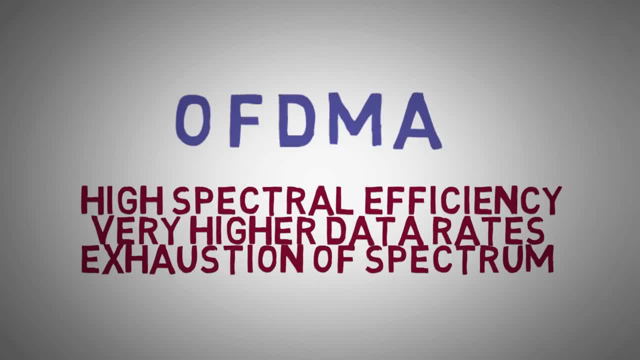 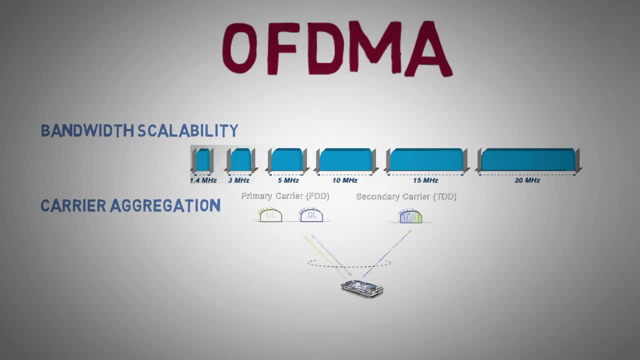 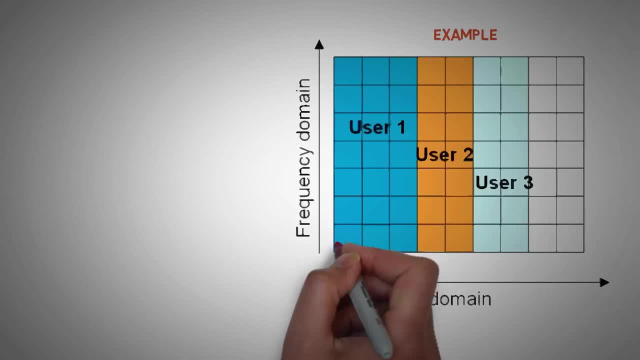 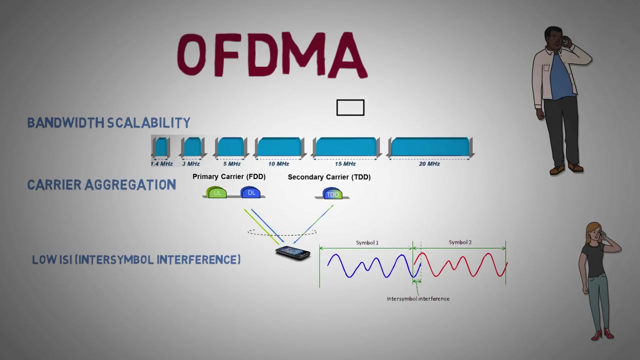 OFDMA uses orthogonal subcarriers equally spaced at 15 kHz. Users are provided a subset of these subcarriers for data transmission. Unlike FDMA or TDMA, OFDMA allows the users to access variable bandwidth depending upon the resource availability. Also, since these subcarriers are orthogonal, there are no guard bands. 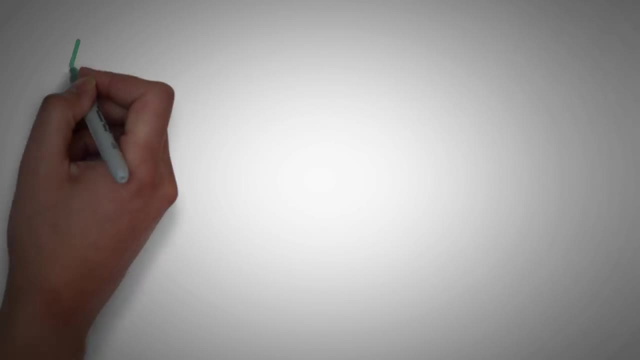 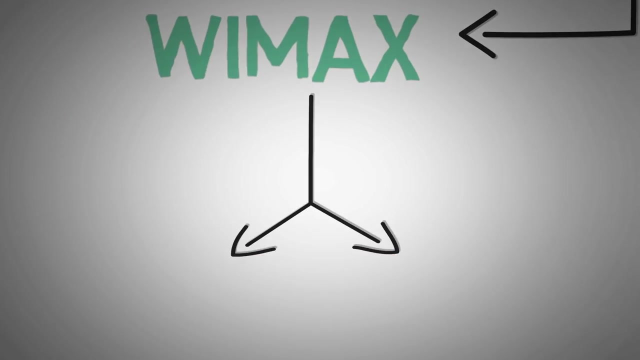 And like WCDMA in the same way, of course, of course, of course I use WCDMA. Thanks for watching and see you next week. bands between them. it was first introduced in Wi-Fi and subsequently in WiMAX by IEEE, but as WiMAX lacked backward compatibility and support for 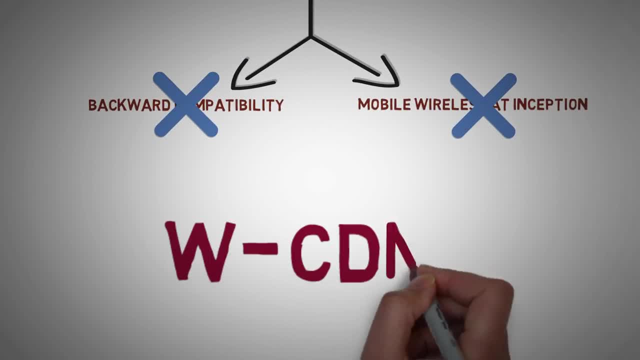 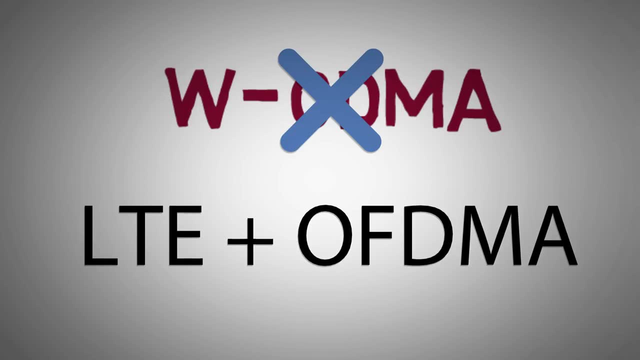 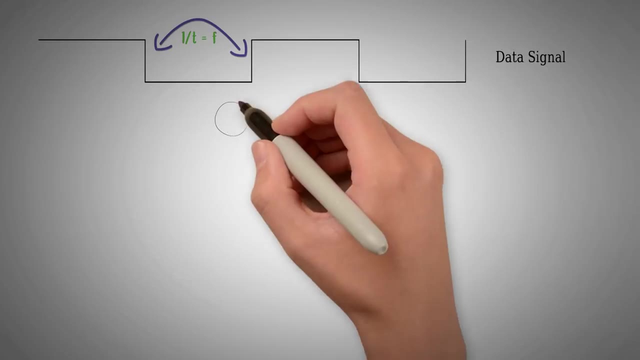 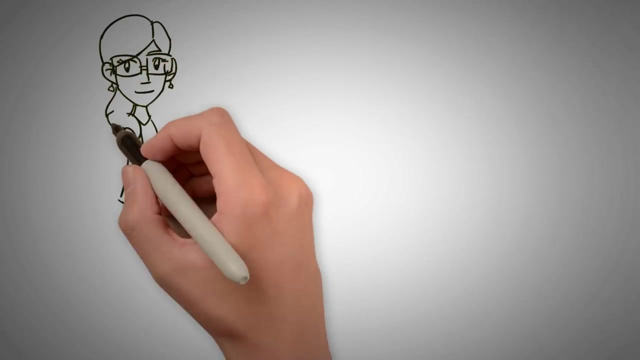 mobile wireless at its inception, operators remain stuck with WCDMA. this changed with the introduction of LTE, which brought OFDMA to the forefront of today's mobile networks. so today we showed what were the different multiple access techniques that were used in various generations of wireless communication. in our next video we will dive deep into OFDMA and SCFDMA. 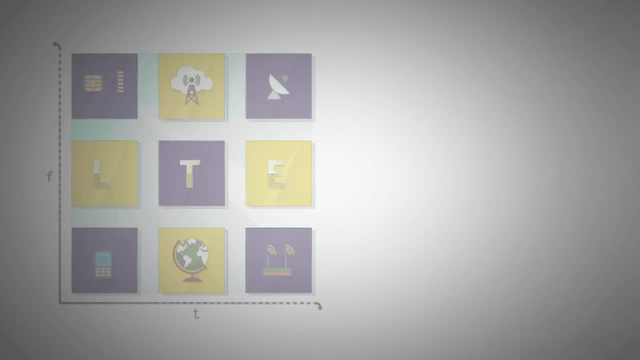 the two pillars of 4G. hope you enjoyed the video. don't forget to subscribe to our channel to stay updated. happy learning.